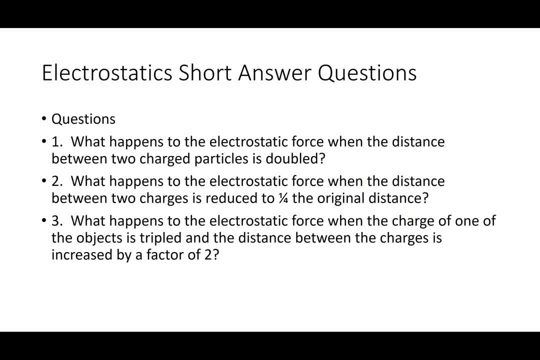 This is Matt Dean, with A Plus College Ready, and today we're going to work some electrostatics practice problems. We're going to start with some short answer questions. What happens to the electrostatic force when the distance between two charged particles is doubled? 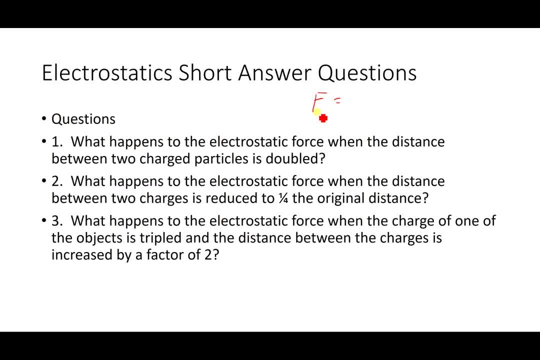 We'll have to use Coulomb's law to guide our thinking here, which is F. sometimes you'll see it written as FE equals K, the Coulomb's constant times charge one times charge two, all over the distance between the charges centers squared. You may see that written as R squared or D squared. 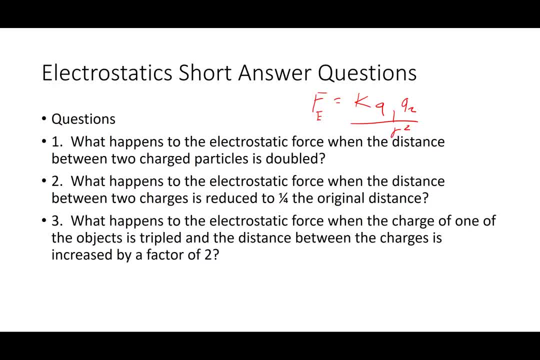 So we want to know what happens to the force when the distance is doubled. So if we double this R we've got to square it. So two squared is going to have given us a four on the bottom of the fraction. I hope that tells you that the new force is going to be one fourth of the original force. 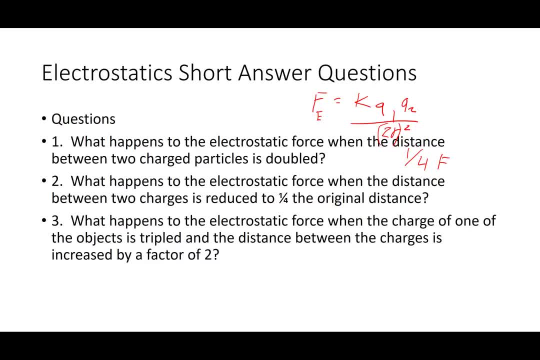 Remember that Coulomb's law and the law of universal gravitation are both inverse square laws. The magnitude of the force varies inversely with the square of the distance between the object centers. Two wants to know what happens to this electrostatic force when the distance is reduced. 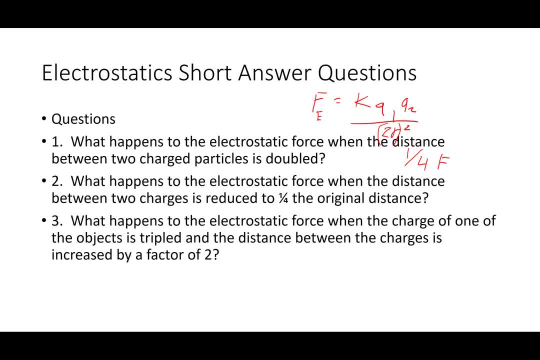 to one fourth the original distance. So again we can use Coulomb's law to guide our thinking. So this time the new distance is one fourth that original distance. We've got to square that one fourth, So that's going to give us one sixteenth on the bottom of. 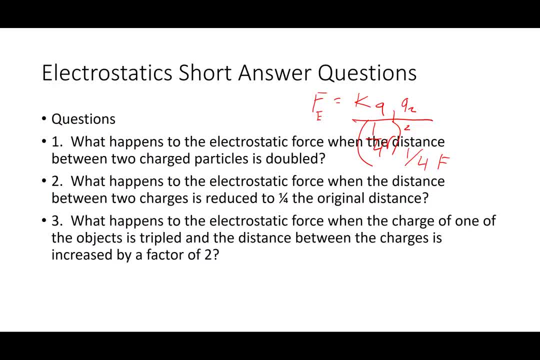 our fraction. Well, when we simplify the fractions, that 16 is going to flip up to the top, And that should tell us that the new force is 16 times the original force. The last one, F, equals K, Q1, Q2 over R squared. We want to know what happens to the force. 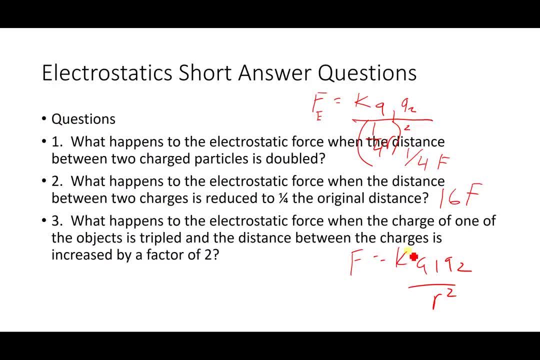 when the charge of one of the objects is tripled. So let's just multiply Q1 times three And the distance between the charges is increased by a factor of two. So let's put a two here. Don't forget to square that two So that three on top is going to increase the force by a magnitude. 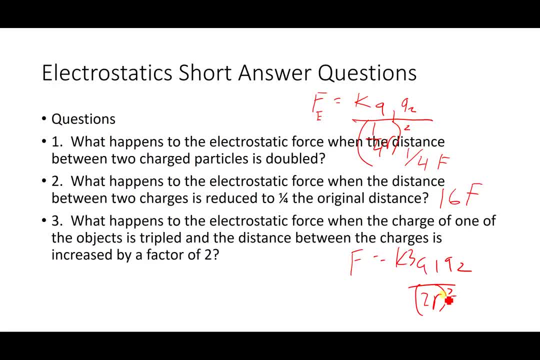 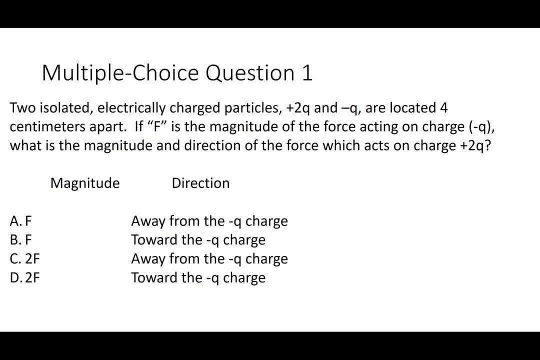 of three, And that two on the bottom is going to decrease the force by a magnitude of four. two squared, So the new force is going to end up being three fourths the size of the original force. So let's move on to multiple choice. question one On multiple choice one. here's what we have. 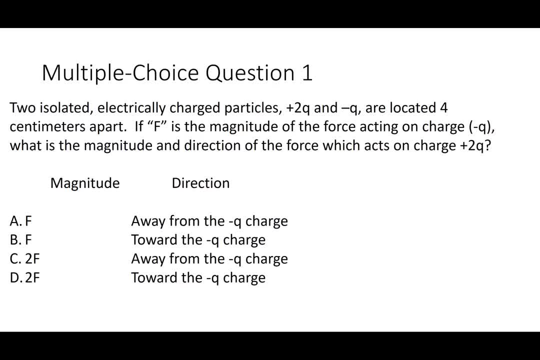 So we have two isolated electrically charged particles. One is plus two Q, One is negative Q. They're located four centimeters apart, That's from center to center, And we want to know if F is the magnitude of the force acting on the negative Q charge. 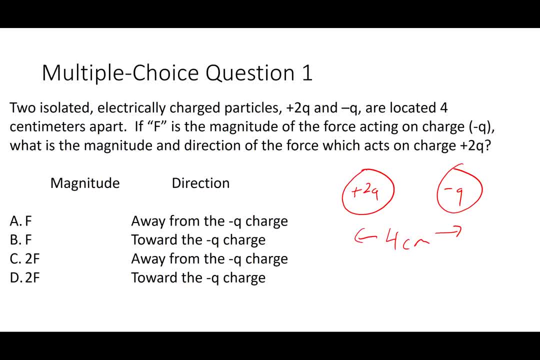 What's the magnitude and direction of the force that acts on charge plus two Q. So we have two isolated electrically charged particles. One is plus two Q, One is negative Q. First of all, the Coulomb law force. Coulomb's law force acts on both charges at the same time. 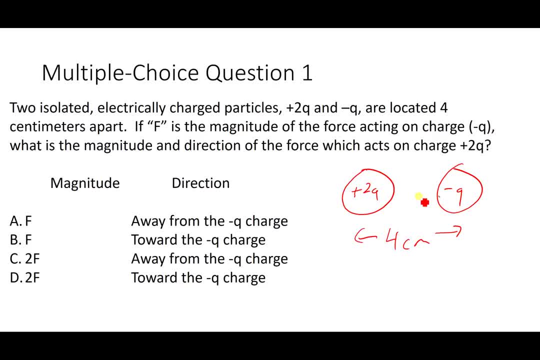 It's a Newton's third law kind of thing. If this charge pulls or pushes on this one, this one pulls or pushes with equal magnitude, but opposite direction. So the magnitude of the force on both charges has to be F. Now what tells you the direction is that. 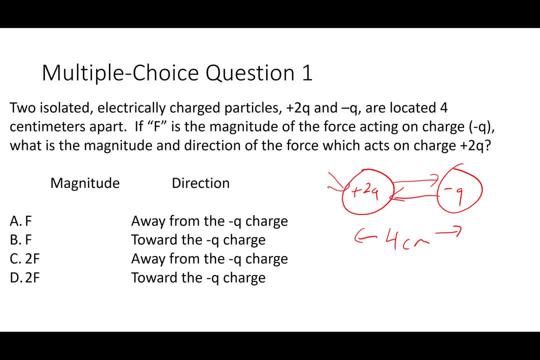 these two charges have opposite signs. This one's a positive, This one's a negative. When Coulomb's law gives you a, a um charges with two opposite signs, the Coulomb's law force is going to be attractive. So the plus two charge is going to get pulled toward the negative one charge. 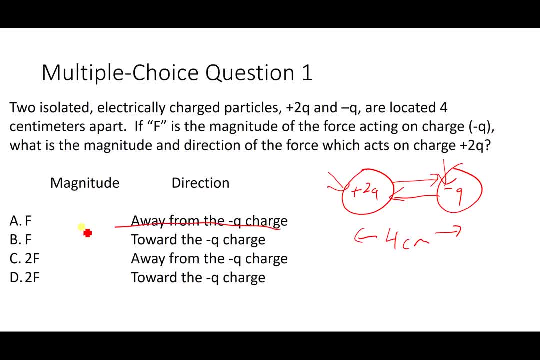 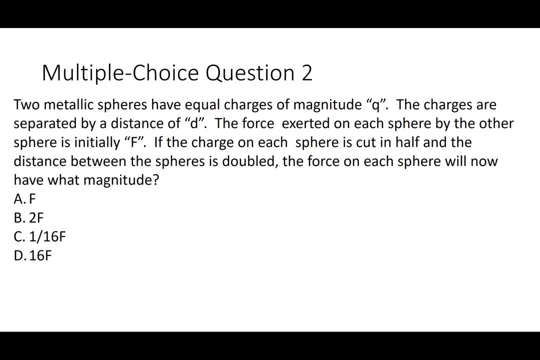 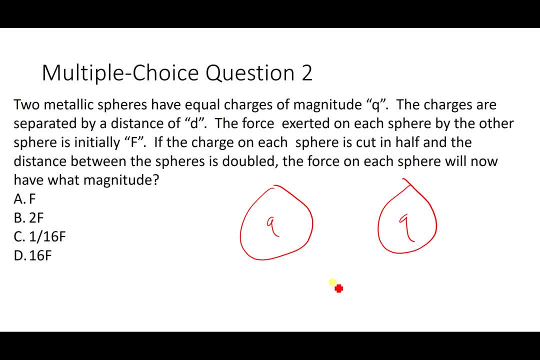 charge Q. The charges are separated by a distance of D. Again, that's center to center. The force exerted on each sphere by the other sphere is initially F. If the charge on each sphere is cut in half and the distance between the spheres is doubled, the new force on each sphere will now: 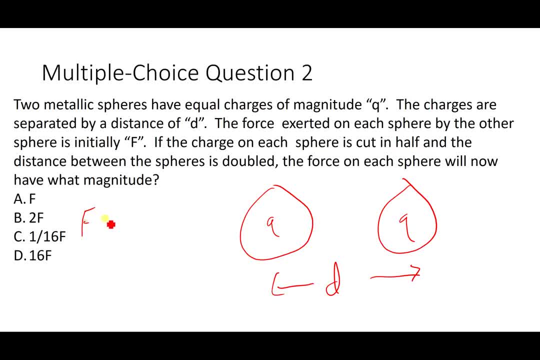 have what magnitude. So we're saying again: use Coulomb's law. We're going to cut charge one in half, We're going to cut charge two in half And we're going to double the distance. Remember we have to square that distance. So the two halves on top are going to end up decreasing our force. 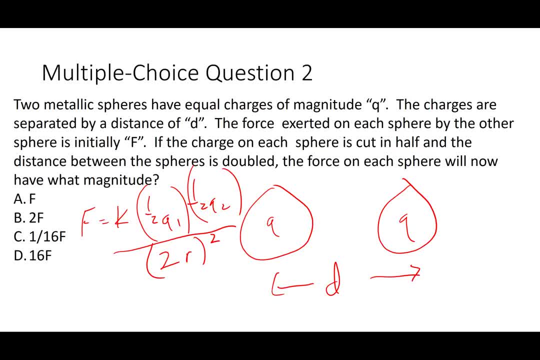 by a magnitude of one fourth. It's going to be one fourth of what it originally was. according to the change on top, The two on the bottom is going to decrease it to another fourth. So if we, if we simplify one fourth on top divided by four on bottom, that gives us a 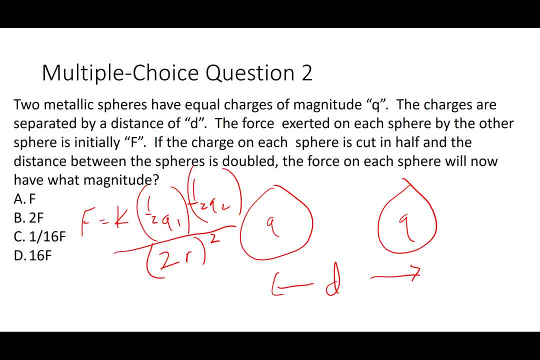 change in the force. So we're going to cut charge two in half And we're going to double the distance. So our answer here is that the new force is going to end up being one sixteenth the size of the original force. So we're looking at answer C. Moving on to question three, Two spheres initially. 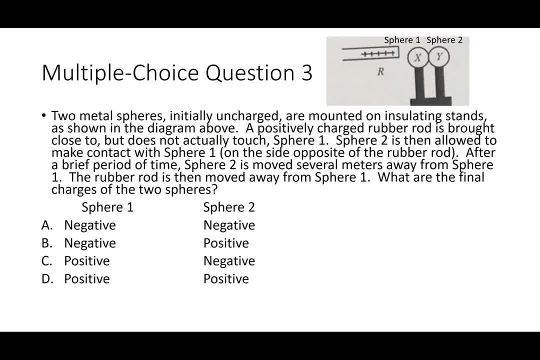 uncharged, are mounted on insulating stands. as shown in the diagram. A positively charged rubber rod is brought close to, but does not actually touch sphere one. Sphere two is then allowed to make contact with sphere one. Sphere two is then allowed to make contact with sphere one. Sphere two is: 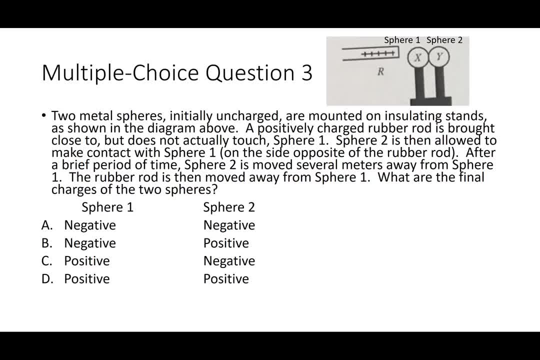 then allowed to make contact with sphere one On the side opposite of the rubber rod. After a brief period of time, sphere two is moved away several meters from sphere one. The rubber rod is then moved away from sphere one. What are the final charges of the two spheres? All right, this. 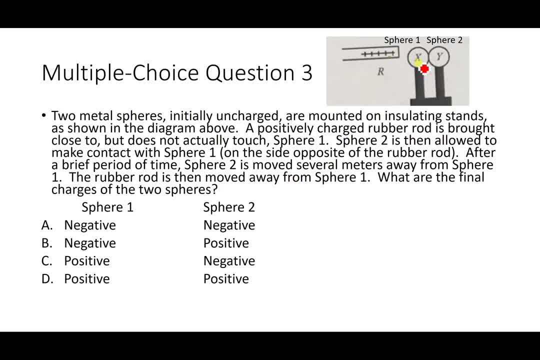 positive rod is going to attract electrons from X over toward this side. When sphere two touches one, this side of X is going to be positive, So it's going to attract electrons from Y over to it and those are then gonna get attracted over toward the ride. So the net. 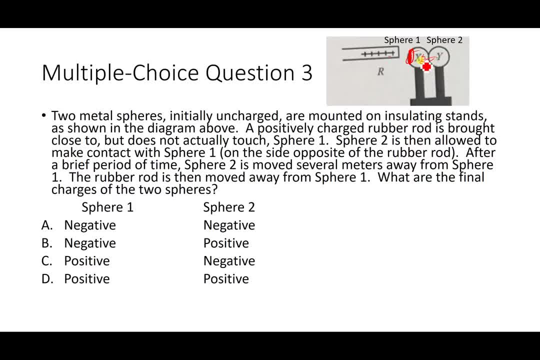 effect is electrons are going to move from Y to X and then over to this side of X. Then, when we move them apart, Y is missing some of the electrons it initially had. X has gained some electrons, so X is going to have an excess of electrons, therefore be negative. Y is going to be 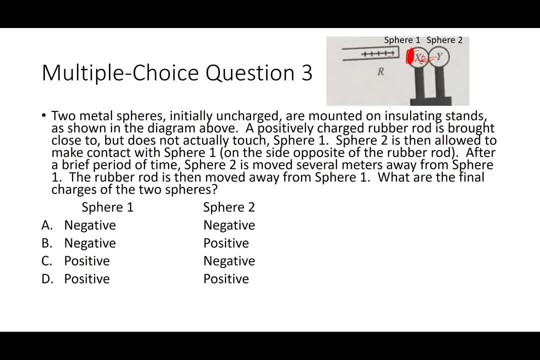 missing some electrons that it initially had. So on the right side of the slide we see one assembly. This is going to be negative, SOaci. Why is that? It's just going be. it's going to be negative. it had to begin with, so it's going to be positive. So our answer here is going to be B. 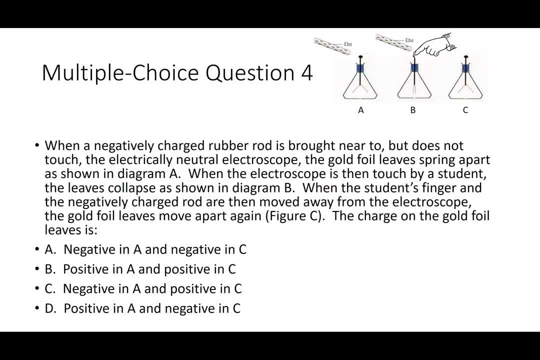 Let's move on to question four. When a negatively charged rubber rod is brought near to but does not touch the electrically neutral electroscope, the gold-foiled leaves spring apart, as shown in diagram A. We see that happening here. When the electroscope is then touched by a student, 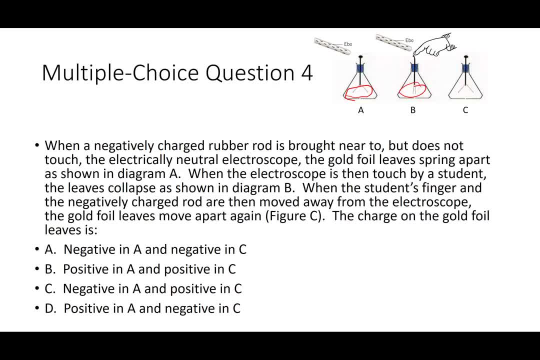 the leaves collapse, as shown in figure B. You can see those leaves are collapsed there. When the student's finger and the negatively charged rod are moved away from the electroscope, the gold-foiled leaves move apart again. We see that happening here. The charge on the gold-foiled 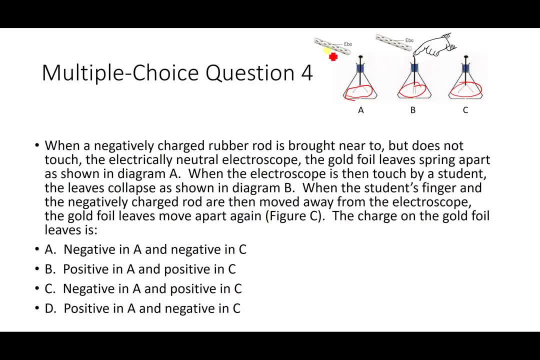 leaves is. Well, here's the thing: This negative rod, when we put it close to this electroscope, it's going to repel the electrons from up here down to those leaves, and those leaves separate because they both have excess nitrogen. 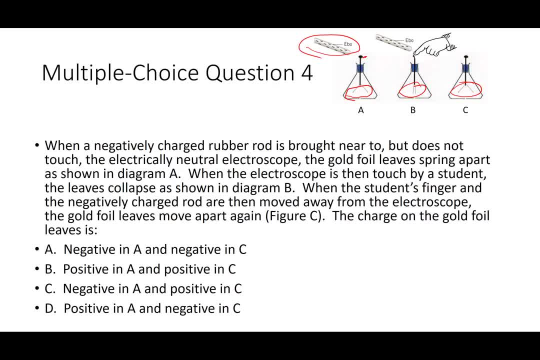 Negative charge. So in A those leaves are negative. In B, when we touch, when the student touches the electroscope, the student's grounding it, which means some of those extra charges are going to be repelled into the student and out of the electroscope. So the electroscope is losing negatives. 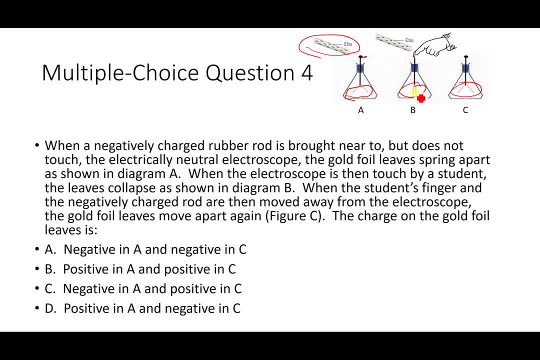 That's why the leaves go back together. The negatives that were down here have now moved into the student. When the student moves back together, the negatives that were down here have now moved into the student. When the student moves the finger and the rod is moved, the leaves go apart again, because 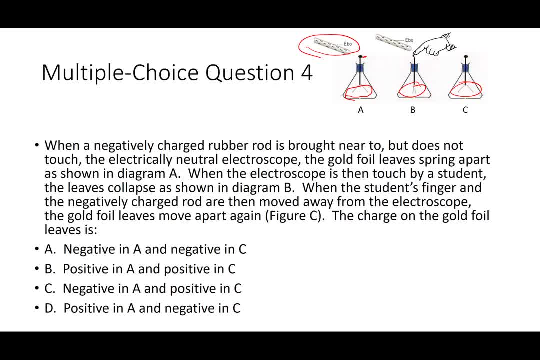 here's the thing: The electroscope is now missing charges. Electrons that it used to have aren't there anymore, which means there's an excess positive charge now, and that's why the leaves go apart, because now both leaves are positively charged. Positive charges repel. 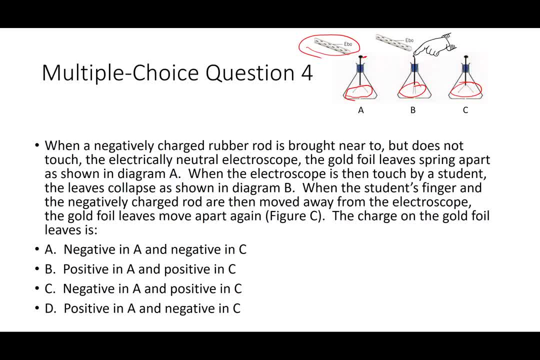 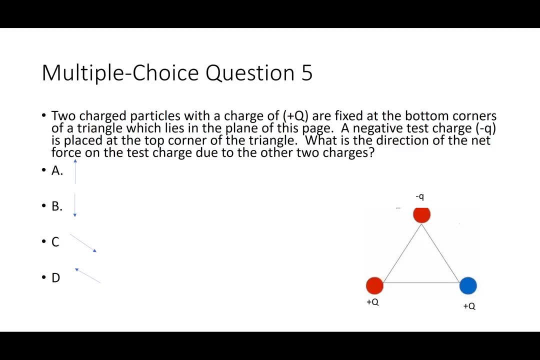 each other. So our answer is: it's negative in A, positive In C. so that's going to be choice C. All right, now we're on question five. Two particles with a charge of plus Q are fixed at the bottom corners of a triangle which lies in the plane of this page. So here and here. 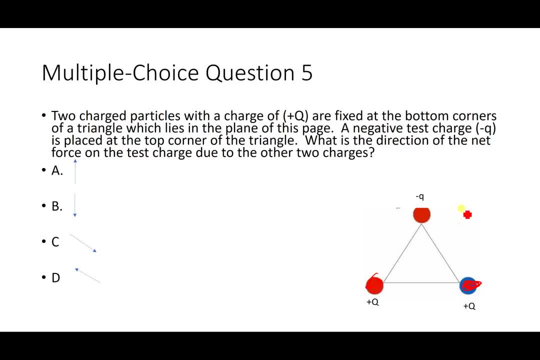 A negative test charge of negative Q is placed at the top corner of the triangle. What is the direction of the net force of the charge? It's the direction of the net force of the charge. A negative force on the test charge is proposed due to the Creo or the current direction. 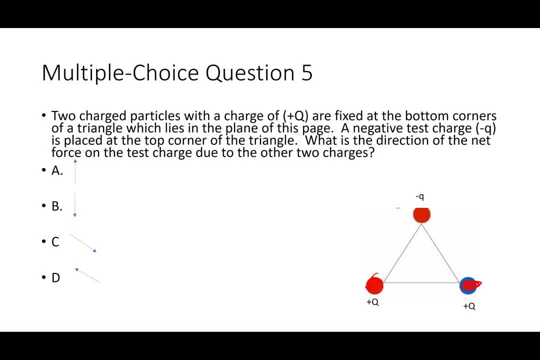 of these two charges pulled from negative and positive list Bs. Well, here's the thing. This charge Qis, is pulling this way on negative Q. This charge is pulling this way on that one. The charges are the same. They're the same distance from. 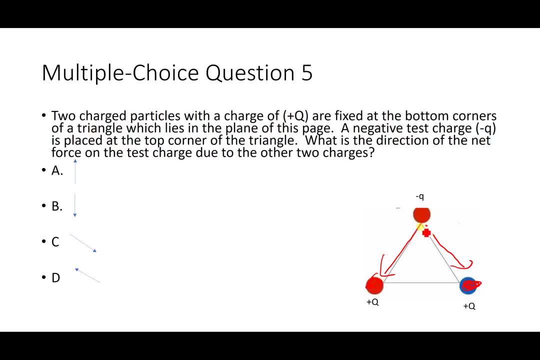 negative Q, which means we could break these charges into two components. Something like this: It can work or it can't work, And this charge is pulling over negative, This charge is pulling down. It's also pulling forward or it's pulling back down. There are back and forth. I hope that you are getting. 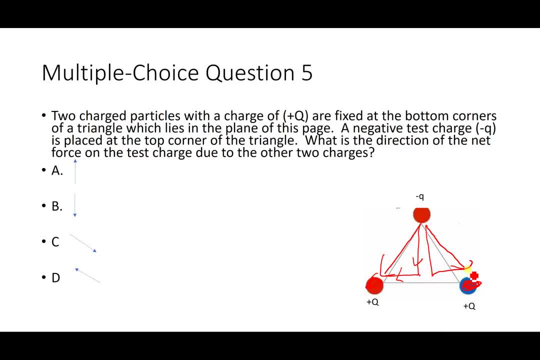 to the left. This charge is pulling down. It's pulling to the right. This left component here and the right component here are equal in size but opposite in direction. They cancel out. These two down components actually add together and double the downward force. 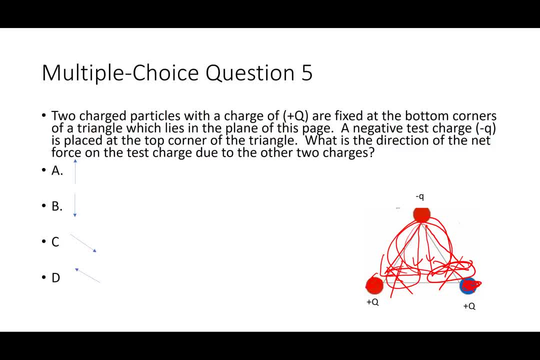 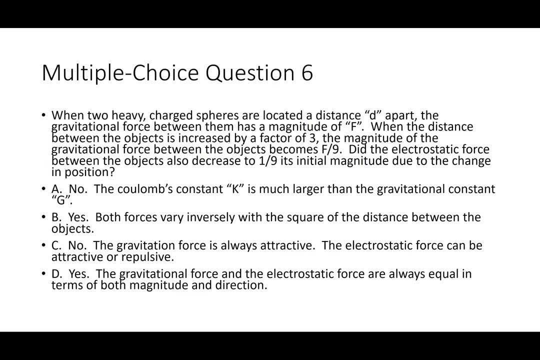 Point being, the net force acting on negative Q is going to be downward. It's going to be attracted to the positive charges. That's answer B. Moving on to six, When two heavy charge spheres are located a distance D apart, the gravitational force between them has a magnitude of F. Here are our spheres: 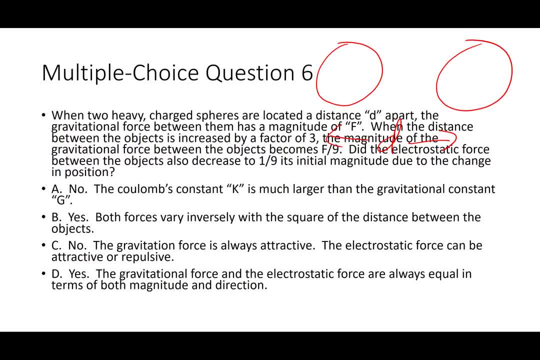 Again, they're distance D apart. When the distance between the objects is increased by a factor of three, the magnitude of F is increased by a factor of three. The magnitude of the gravitational force between the objects becomes F over nine. Did the electrostatic force between the objects also decrease to one-ninth its initial magnitude? 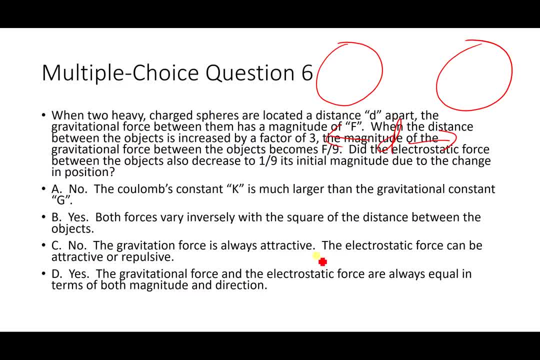 due to the change in position. What you've got to remember is that the law of universal gravitation looks like this: G times M1, M2 over R squared. When we increase this distance by a factor of three, the gravitational force is now one-ninth of what it originally was. 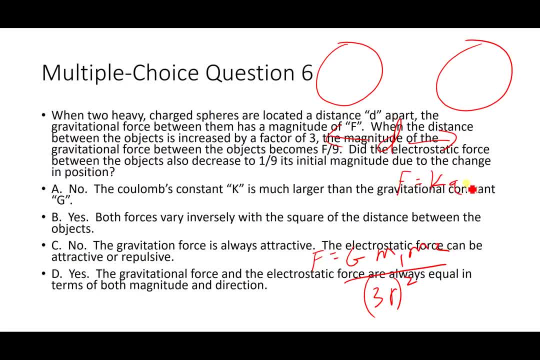 Remember that Coulomb's law looks almost just like that. It's also an inverse square law. When this distance becomes increased by a factor of three, that three gets squared and the new force is one-ninth of the original force. The answer is yes. It's because they're both inverse square laws, which is essentially what 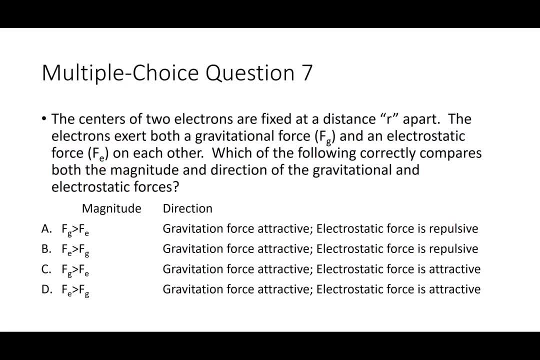 choice B tells us: All right. here's multiple choice question seven. The centers of two electrons are fixed and distance R apart. The electrons exert both a gravitational force and an electrostatic force on each other. Which of the following correctly compares both the magnitude and the direction of the gravitational and electrostatic? 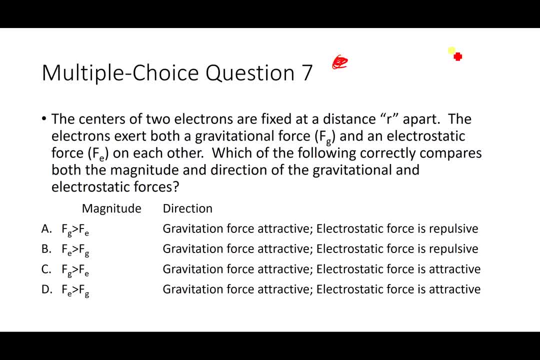 forces. So here are our electrons. Remember electrons are negative. The gravitational force is going to attract anything else with mass. So the gravitational force is going to try to pull these two objects together. It's attractive. The electrostatic force, on the other hand. 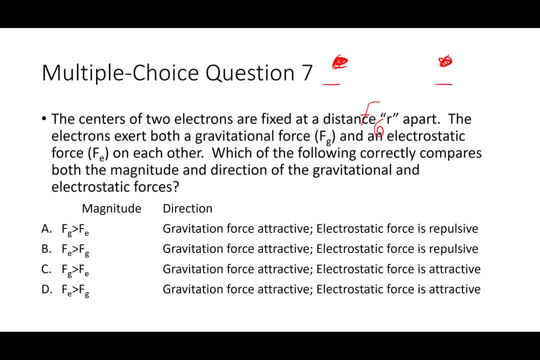 since they're both negative, is going to be a repulsive force. It's going to try to push them apart. So we know gravity is attractive and in this case, electrostatic is repulsive. So that means we either got to have answer A. 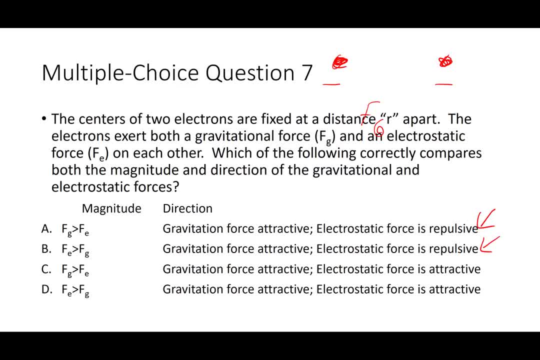 or answer B. Now here's the thing. Remember our two equations for gravitational force and electrostatic force. look almost identical, But what's different is the universal gravitation constant in K. K is equal to a factor of nine times 10 to the ninth, Whereas G has a value of 6.67 times. 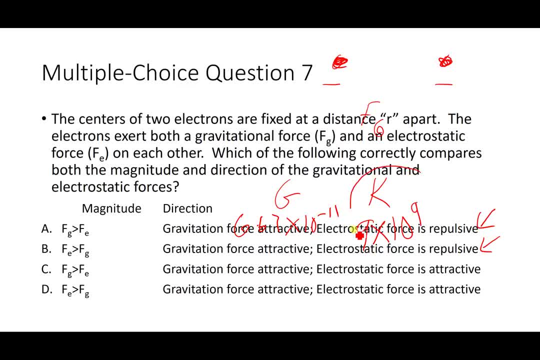 10 to the minus 11.. Because K is so much greater- a factor of almost like a magnitude of 20 times greater than G, the electrostatic force between charged objects is almost always going to be much greater than the gravitational force. So what that's telling me is that the electric force is going 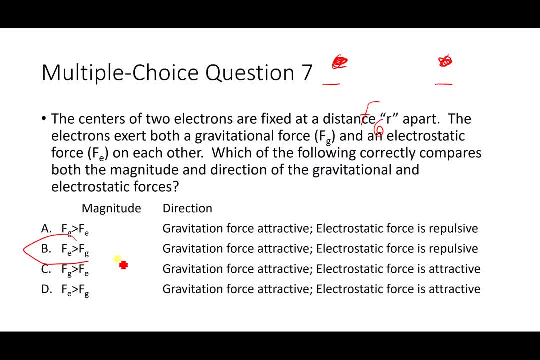 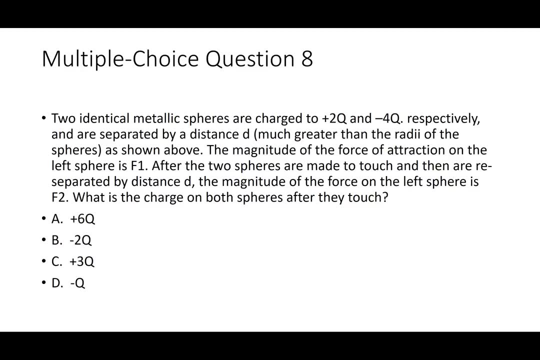 to be bigger than the gravitational force. So I'm looking at answer B as my correct answer. All right, let's move on. Let's go on and look at questions number eight. Two identical metallic spheres are charged to two plus 2 q. 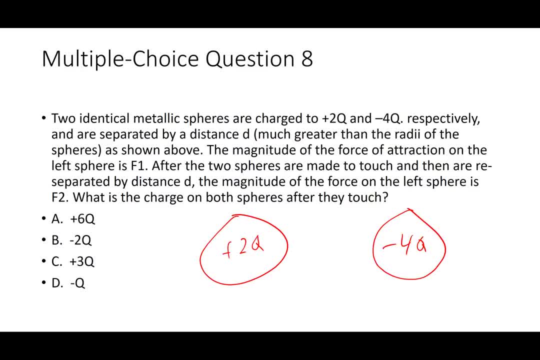 and negative four q, And they're separated by a distance d. The magnitude of the force of attraction on the left sphere is F1.. After the two spheres are made to touch, and then our receptionmom will be starting over again, then twoército spirituales, initially different from direct attraction and then are separated by distance d. The magnitude of the force of attraction on the left sphere is F1.. After the two spheres are made to touch, and then our recipient will be at the center of the sphere, is considered 60 degrees F1. we hit, enter and then we attacked to the left". 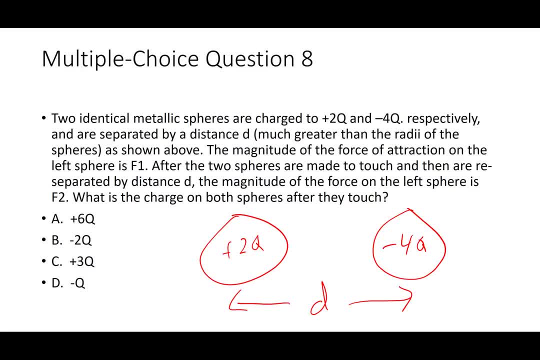 re-separated by a distance d. The magnitude of the force on the left sphere is F2.. What is the charge on both spheres after they touch? When you touch two identical spheres together, they're going to equally share the charge, So the way to work this problem is just. 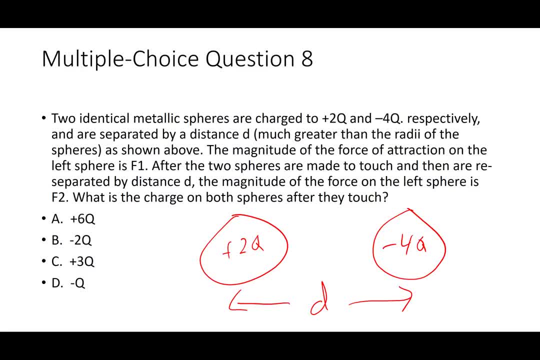 to take plus 2 plus minus 4.. Add those together. Plus 2 minus 4 gives you negative 2 and that charge is going to be divided amongst two spheres. So you're going to go the negative 2 total charge divided by 2.. So each sphere is going to end up with a charge of negative q, negative 1q. 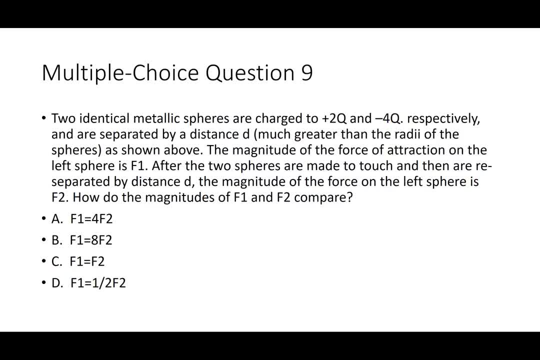 So we're looking at d, Let's go on and do number 9.. Similar question, same idea. This time we want to know, after the two spheres are made to touch and then re-separated by d, the magnitude of the force on the left sphere is F2.. What is the force on the left sphere after they touch, When you? 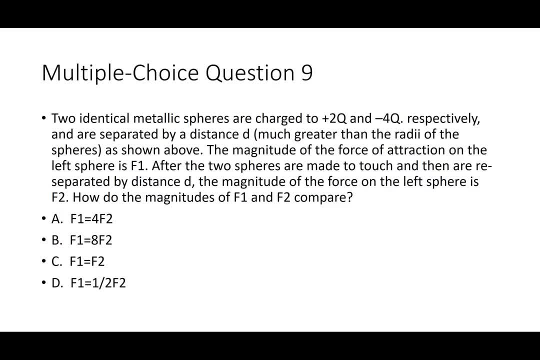 re-separated by d, the magnitude of the force on the left sphere is F2.. How did the magnitudes of F1 and F2 compare? All right, so what we ended up doing, we started off. let's write out what we started off with. So, for F1, we had a situation where we had k times plus 2q times minus 4q. 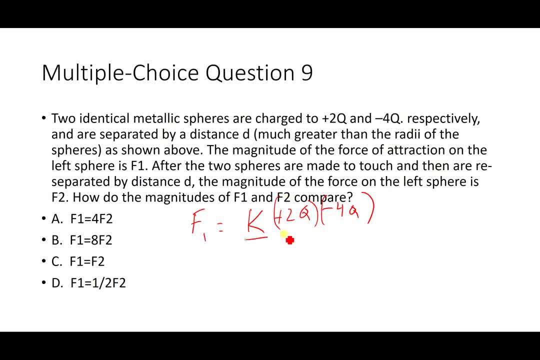 all over d squared For F2, once we let them touch now I have k times negative q times negative q all over d squared. What I want you to see about these two equations is that they have in common k, d and q. 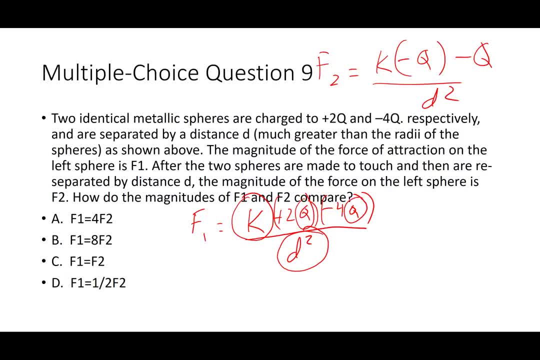 Or q squared. So I'm just going to call that quantity kq squared over d squared. I'm going to call that just x. So if I do that, I can rewrite this equation as negative 8x and I can rewrite the 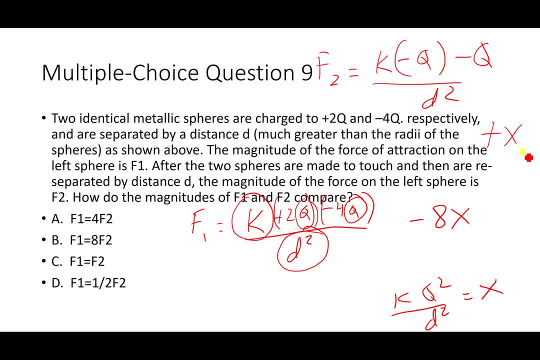 equation on top as plus x. So what I'm hoping that tells you is that F1, F1 is essentially 8 times bigger in magnitude than F2.. All right, so let's look at the free response question now. So we have three particles that are fixed in place in a horizontal plane as 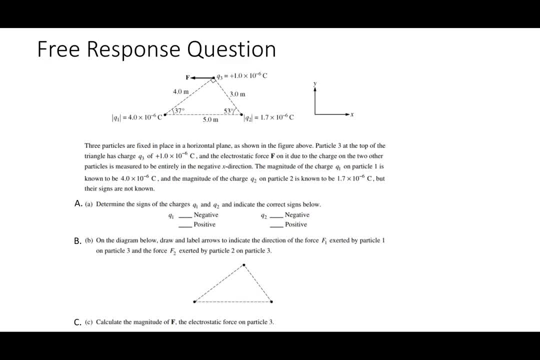 shown in the figure above, Particle 3 at the top of the triangle has a charge of 1 times 10 to the minus 6 coulombs And there's an electrostatic force at the top of the triangle And there's an 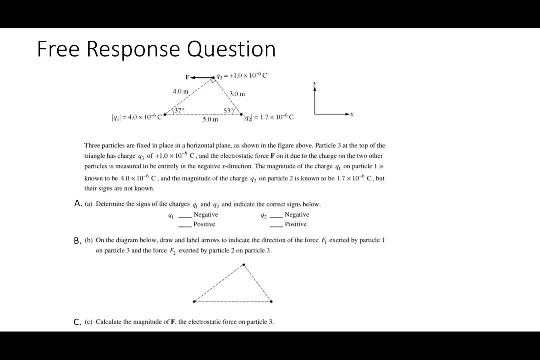 electrostatic force on it due to the other two charges that pushes entirely in the negative x direction. The magnitude of the charge q1 on particle 1 is 4 times 10 to the minus 6.. And the magnitude of the charge q2 on particle 2 is known to be of 1 times 10 to the minus 6, but their 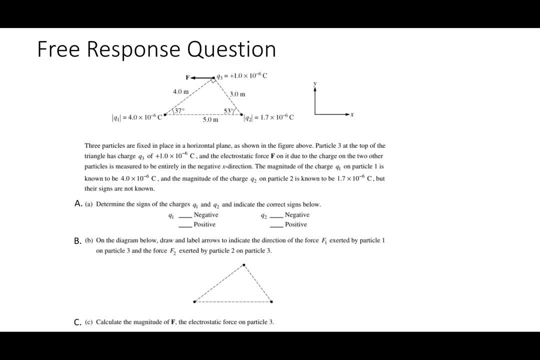 signs are not known. Determine the signs of q1 and q2 and indicate the correct signs below. All right, since the net force acting on q3 is completely in the x direction, here's what we've got to think about. This force is going to have to be positive. q2 is going to 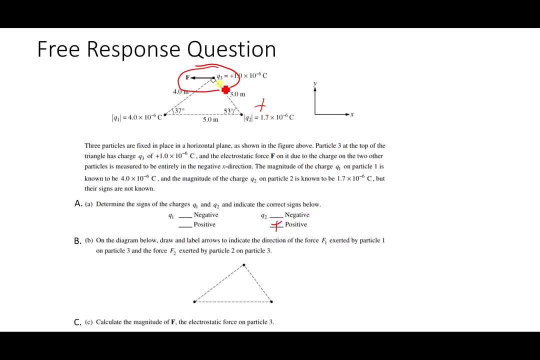 have to be positive because it's repelling q1. It has a component that's pushing this way And therefore it would also have a component that was pushing it up q1,. on the other hand, it has to be negative because it's attracting the force. It has a 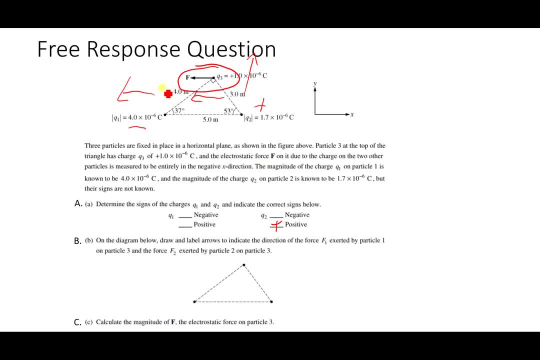 component that's pulling in the x direction. It also has a component that's pulling in the x direction. It also has a component that's pulling down. So the horizontal components of both of the forces add together The negative component- downward component here- and the positive component here. 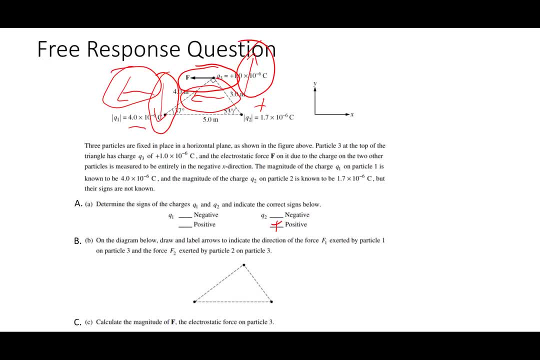 cancel out. That's how we end up with a net force in the horizontal direction. All right, let's move on to b. On the diagram below, draw and label arrows to indicate the direction of the force f1 exerted on the x direction. This is the direction of the force f1 exerted on the x direction. 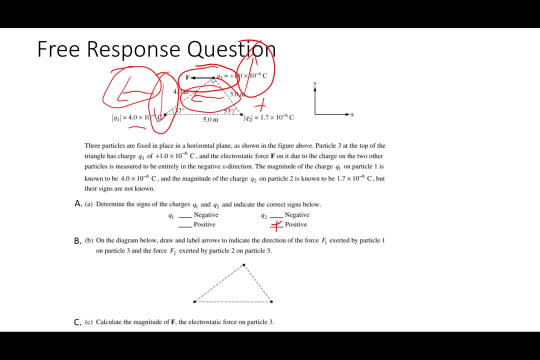 This is the direction of the force f2 exerted by particle 1 on particle 3, and the force f2 exerted by particle 2 on particle 3.. All right, well, here's particle 3.. Here's particle 1.. Since particle 1 is negative, the force it's going to exert. 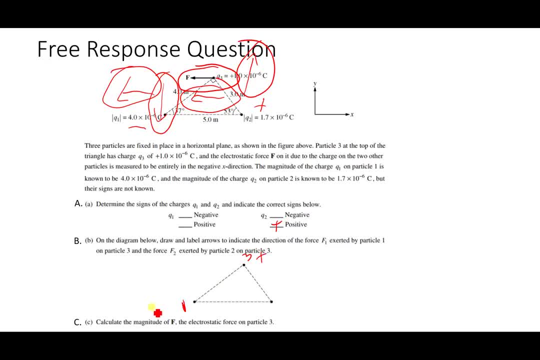 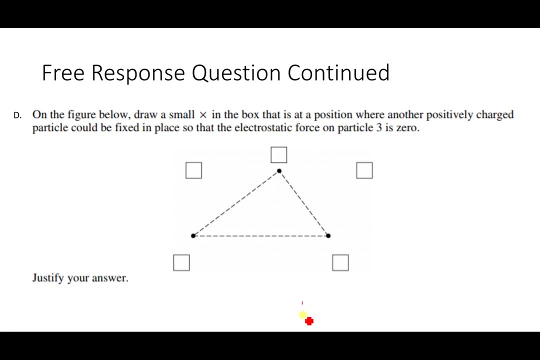 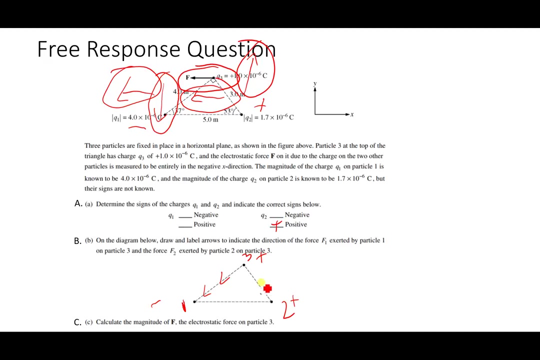 since this is positive, it's going to be an attractive force, so it's going to go in that direction. On the other hand, particle 2 is positive and since it's positive, it's going to be pushing away, and it's going to push away in this direction. 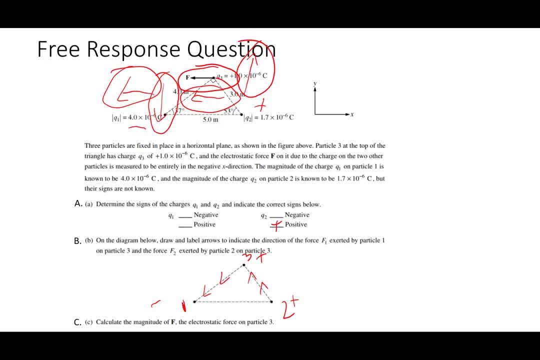 Part. we want to calculate the magnitude f of the electrostatic force on particle 3.. All right, to do that. we're going to have to calculate the Coulomb's force between particle one and particle three, and also between particle two and three. 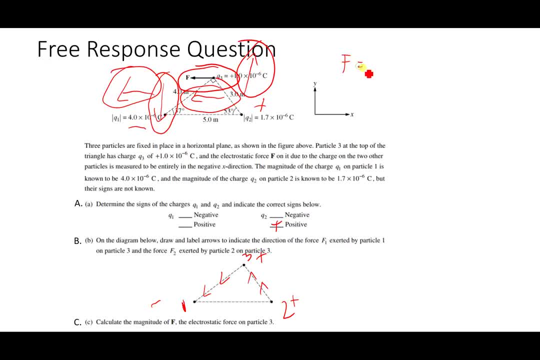 So for particle one and three we're gonna say F equals K. I'm gonna leave off the units on this just to make it not as messy. That's K nine times 10 to the ninth times Q1,. four times 10 to the minus six. 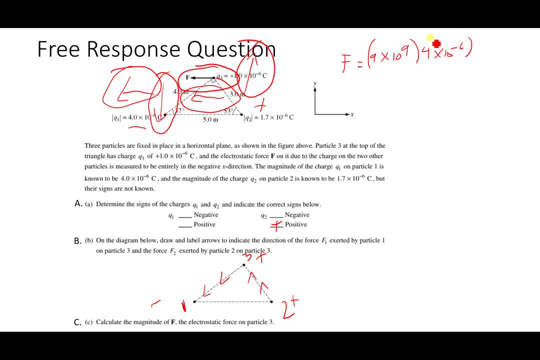 to the minus six times Q3, which is one times 10 to the minus six, all over the distance squared. All right, we calculate that out and that comes out to be 2.25 times 10 to the minus three newtons. 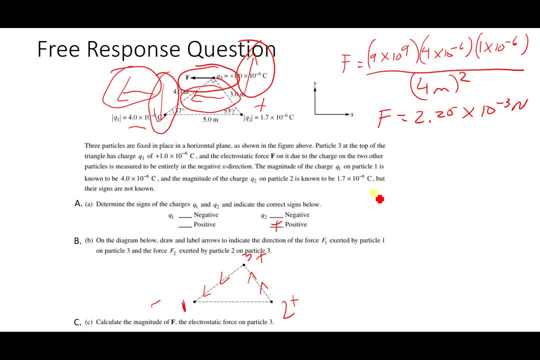 We need to do the same thing for the force of Q2 on Q3.. So F equals K times Q2 times Q1, all over the distance. squared The distance, there is three, And that force comes out to be 1.7 times 10 to the minus three. 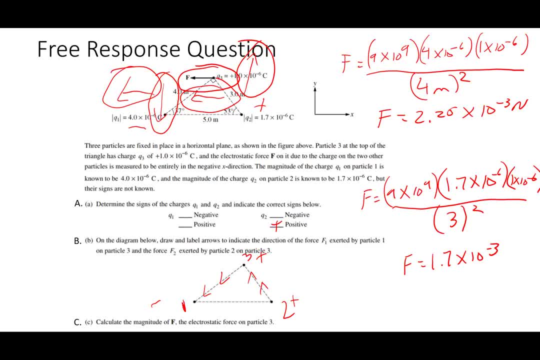 And that force comes out to be 1.7 times 10 to the minus three, And that force comes out to be 1.7 times 10 to the minus three. All right, so what I need to do now is I need to add these two forces together. 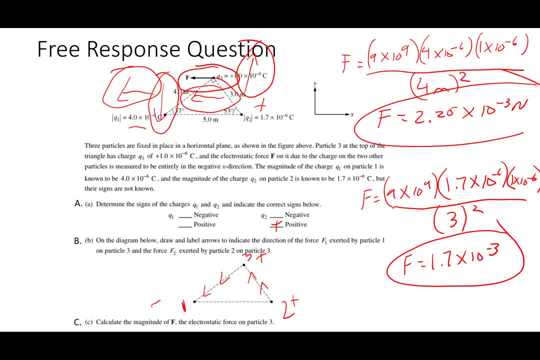 The problem is they're acting in different directions. They're vectors, So what I'm gonna do to add them together is, first of all, I'm gonna break them into components. So this top one is a force that's acting between Q1 and Q3.